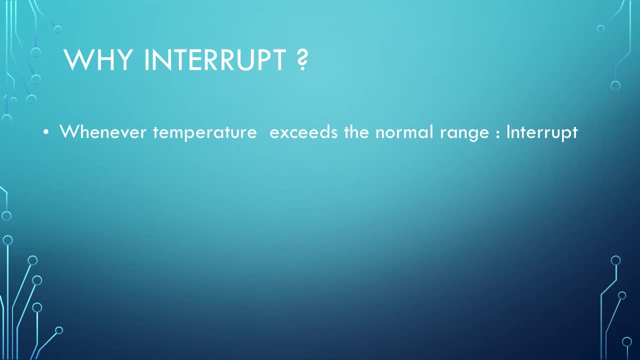 In this particular example, whenever temperature exceeds the normal range, it is to be interrupted. So the processor is continuously monitoring and comparing the temperature. When the temperature is in range, processor is working normally And when the temperature exceeds the default temperature range, it is interrupted. 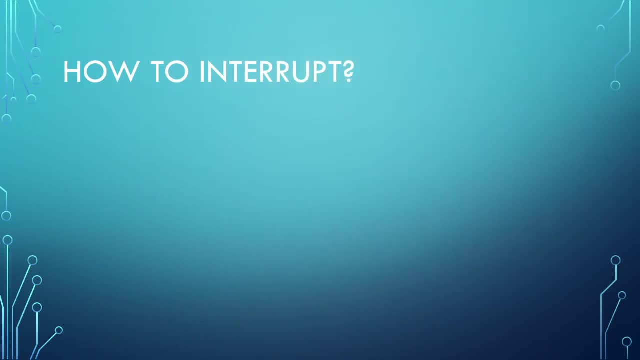 Now how the processor is interrupted. Well, it is done in two ways. First is it can be interrupted on the pin of the processor- that is called hardware interrupts. or it can be done through writing specific instruction in the program and that is termed as software interrupt. 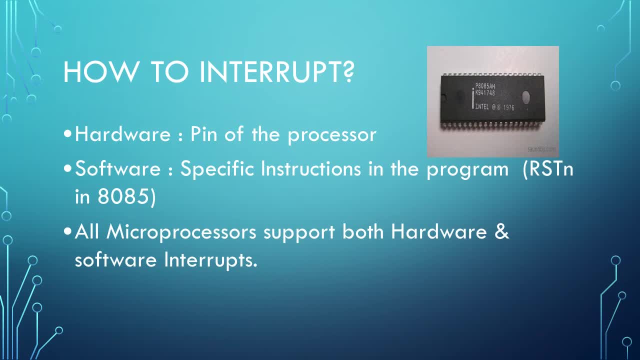 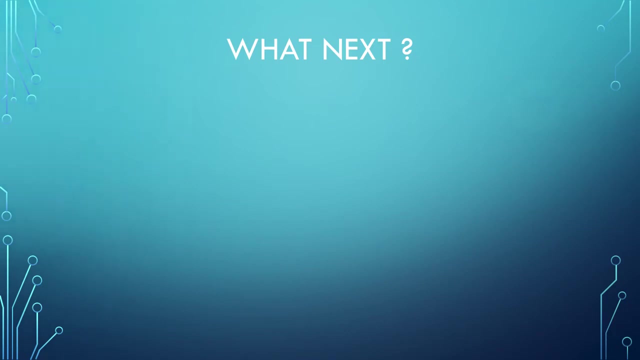 All the processors supports both hardware as well as software interrupt. In our example, we will have software interrupt as the comparing temperature program will give response. Now, when the processor is interrupted, what is to be done? Well, every interrupt, each interrupt, is having two parameters associated with it. First is the name or the number of the 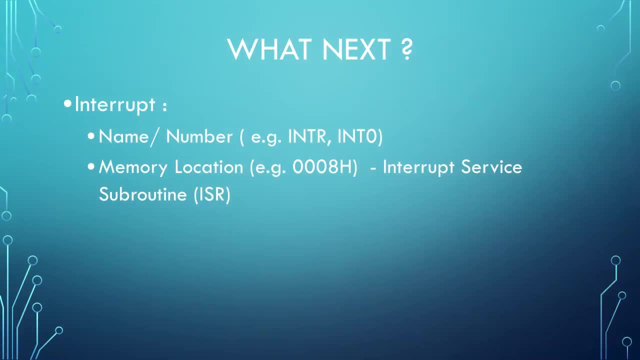 interrupt, by which the processor recognizes the interrupt, and second is the memory location. Whenever an interrupt comes, microprocessor has to go to some memory location to serve interrupt service subroutine. So these are the two parameters associated with the interrupt. So in case of our example we have the main program, which is the normal working. 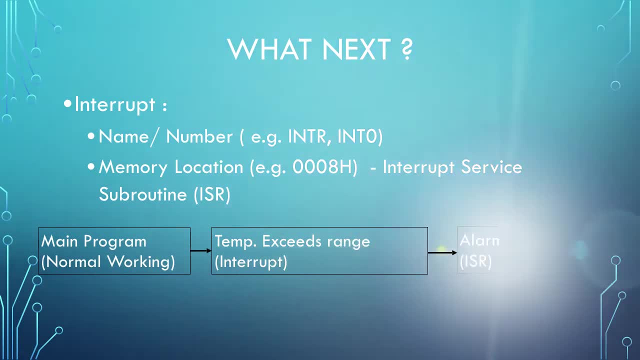 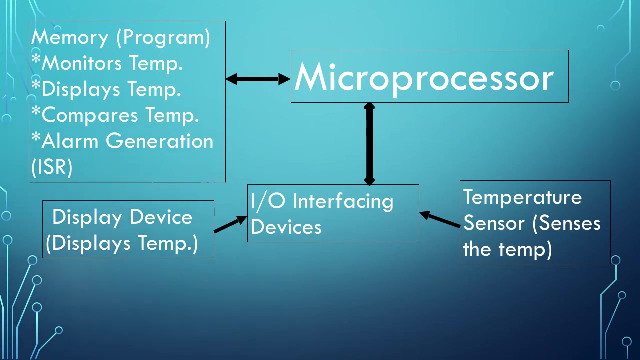 Whenever temperature exceeds the range, the processor is interrupted. and what processor? goes to a service subroutine where it generates an alarm indicating that temperature has exceeded its given range. So again, we have the same setup. we have added one more block to the setup, So the setup. 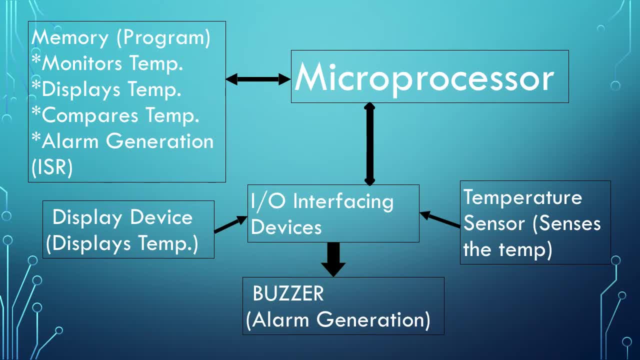 completes this block is of alarm generation. So here microprocessor is monitoring the temperature through sensors, it is displaying the temperature on the display devices, it is comparing the temperature internally and whenever the temperature exceeds the range, microprocessor is interrupted it goes to alarm generation subroutine. 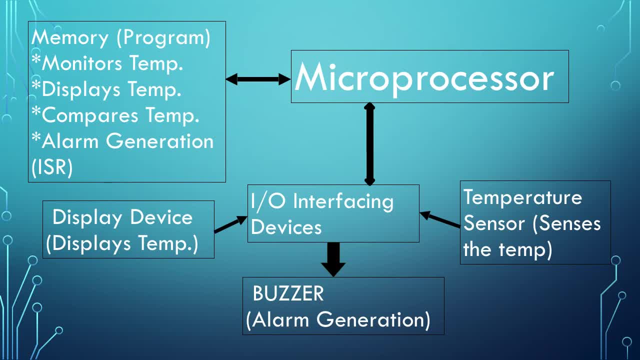 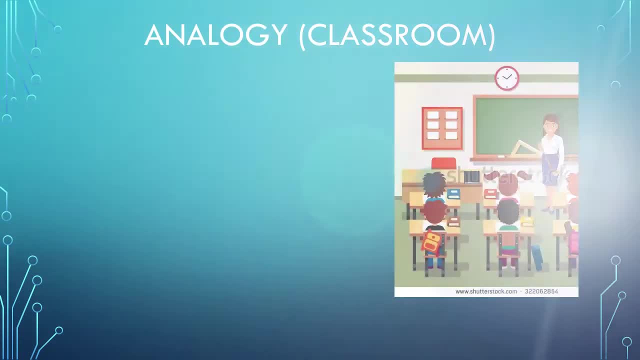 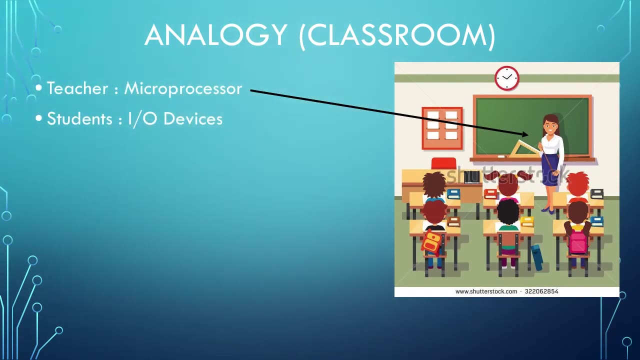 So this is the process of the interruption and it generates an alarm and the buzzer rings. We can understand interrupts with an analogy of classroom Say: we are in a classroom, the teacher is the microprocessor, The students are the input output devices. 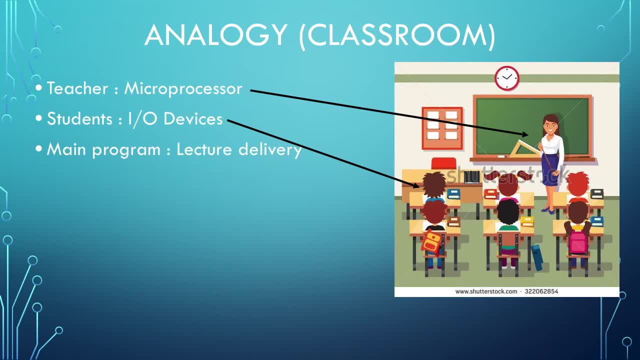 The normal working of the processor is the lecture delivery by the teacher and how the interrupt is generated. Interrupt is generated by the speaker- the speaker has enough stretcher and so it starts- is generated by input output devices, and they are generated when a student raises the hand. 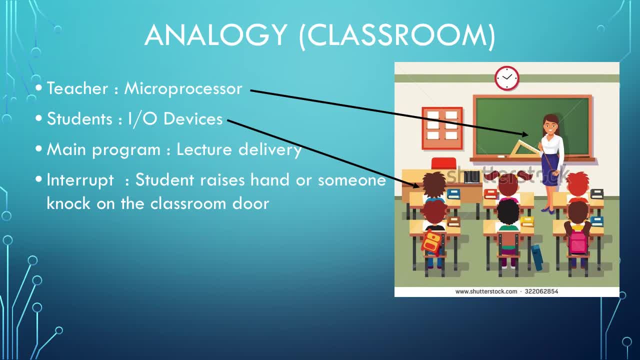 or someone knocks at the door. These are the interrupts to the normal working of the teacher. and what is the subroutine? The teacher will stop delivering the lecture and it will respond to the student or to the knock on the door, and that is analogous to interrupt service subroutine. 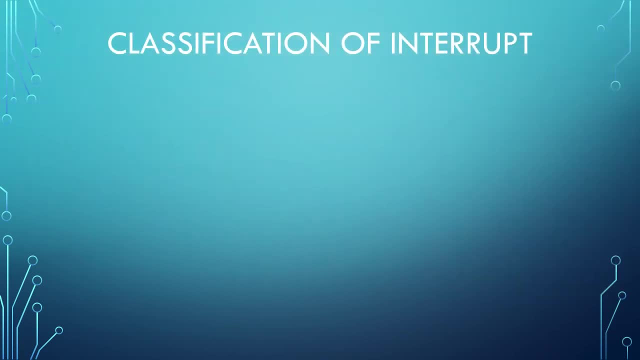 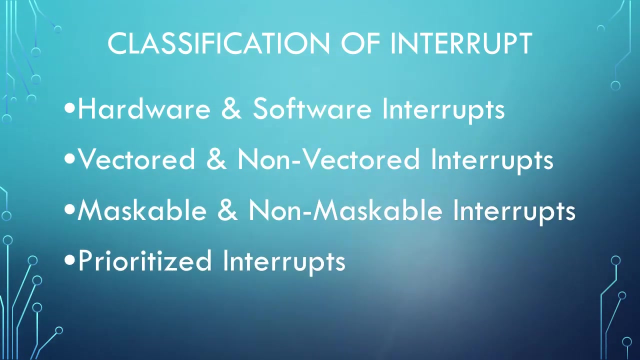 Now we have discussed the concept of the interrupt and we will see the different classification or different types of the interrupt. We have hardware and software interrupts, vectored and non-vectored interrupt, maskable, non-maskable interrupt and prioritized interrupt. 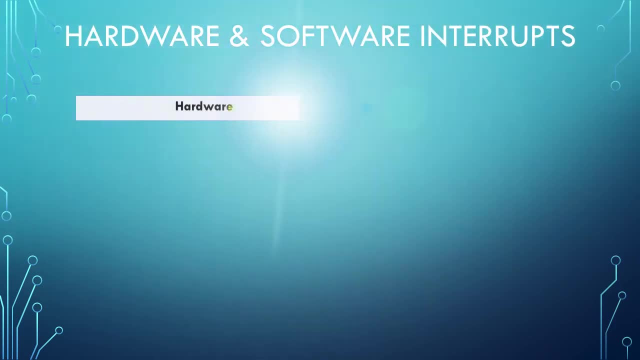 We will discuss them one by one. First is the hardware and software interrupts. Hardware interrupts are generated by the I-O devices or hardware. as I told you earlier, it comes from the I-O devices. Hardware interrupts are generated by the I-O devices or hardware. as 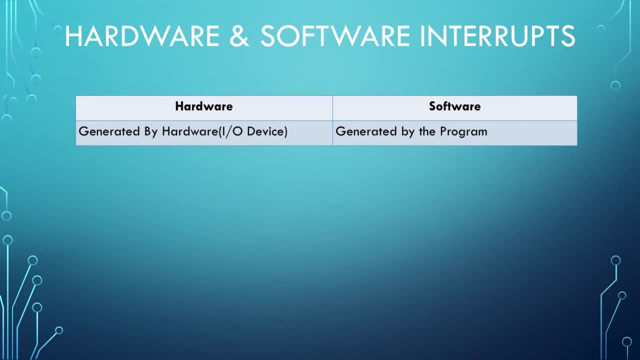 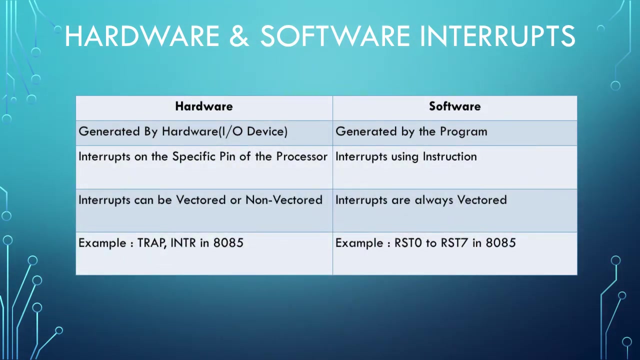 on the pin of the processor, whereas software interrupts are generated by the program. The hardware interrupts come on specific pin of the processor and software interrupts are generated writing the instruction in programs. Hardware interrupts can be vectored or non-vectored, but software interrupts are always vectored. The examples in case of 8085, TRAP and INTR are: 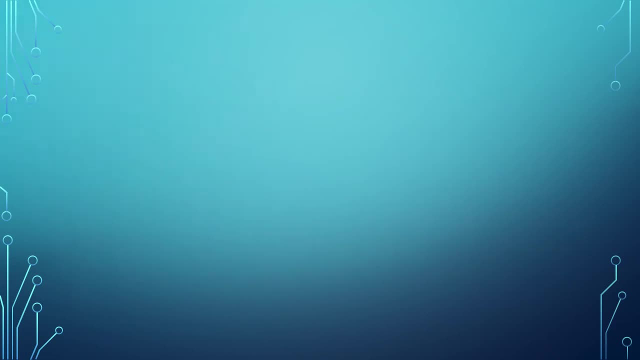 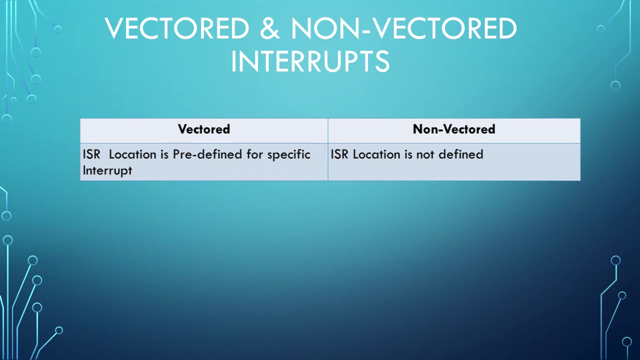 hardware interrupts, whereas RST0 to RST0 are hardware interrupts. Now we used the term vectored in the last slide. What is vectored interrupt? Vector specifies the location. So when the location is predefined in the IC, in the processor, the interrupt is called. 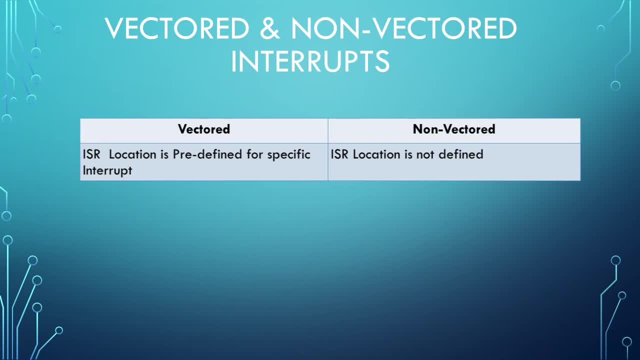 vector interrupt, but if the location is not defined, the interrupt is a non-vectored interrupt. In case of vector interrupt, when the interrupt comes, microprocessor automatically jumps to the predefined location. But in case of non-vectored interrupt, microprocessor gives acknowledgment signal, which is used. 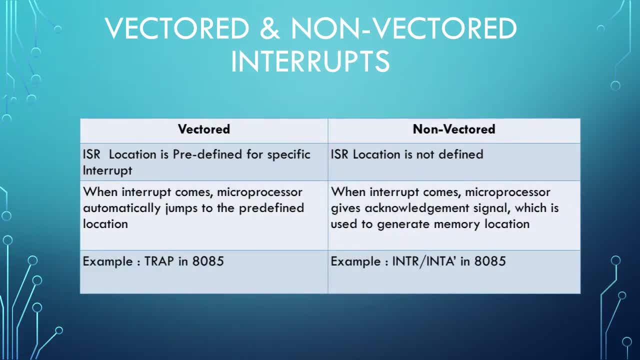 to generate memory location. Examples are: TRAP, in case of 8085, is a vectored interrupt, whereas INTR is non-vectored, and in response to INTR, 8085 generates INTA bar. Now we come to maskable and non-maskable interrupts. 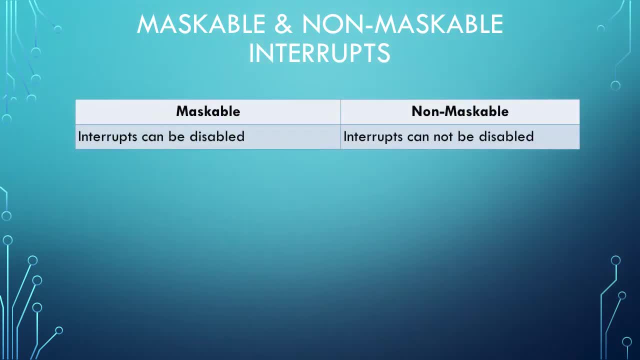 Maskable interrupts mean the interrupts which can be disabled, and non-maskable means the interrupts which cannot be disabled. Disable means when the interrupt comes, and if we disable it it will become pending and microvisor will serve it later. And if the interrupt is non-maskable, if the interrupt comes the microvisor has to serve. 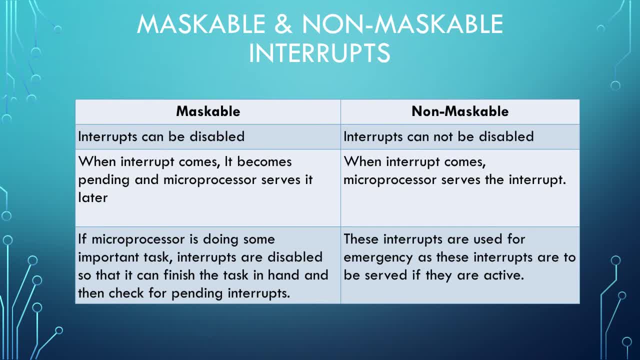 that interrupt Maskable feature is used when microvisor is doing some important task, Then we can disable the interrupt and after finishing the task in hand, microvisor can check for pending interrupt and then serve that interrupt. But non-maskable interrupts. they are used for emergency purposes, as whenever these interrupts 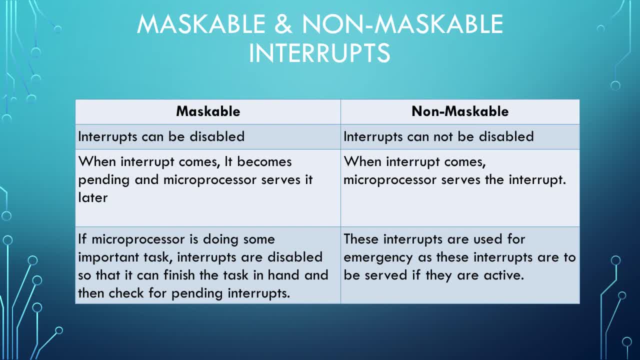 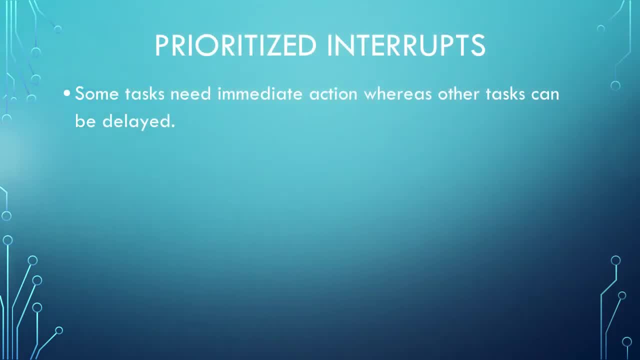 comes, they are to be served. They are active all the time. Now some tasks need immediate attention whereas other tasks can be delayed, So interrupts are prioritized. They follow priority structure. So whenever we have more than one interrupt coming to the process, 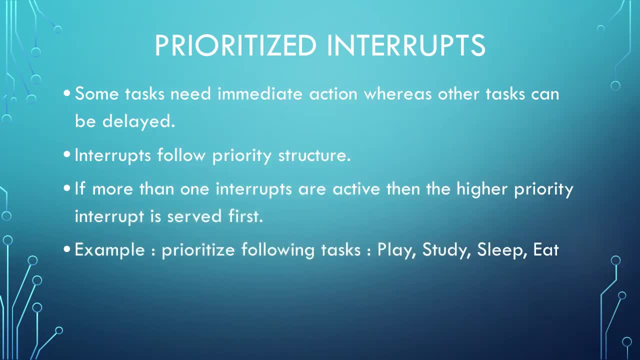 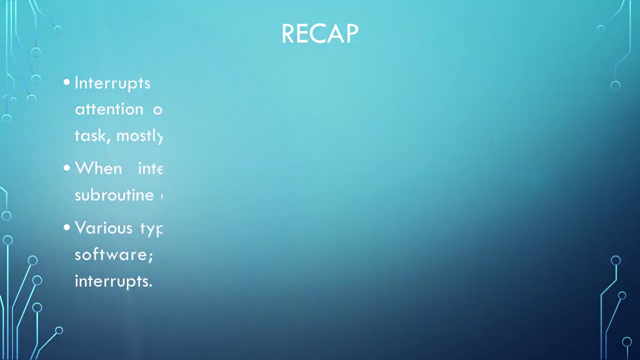 Then higher priority interrupt will be served. This can be analogous to prioritize the following tasks like playing, studying, sleeping and eating. We can prioritize the task. Similarly, microprocessor prioritizes the interrupts. Now a quick recap. Interrupts are hardware or software signals which are used to draw the attention of the 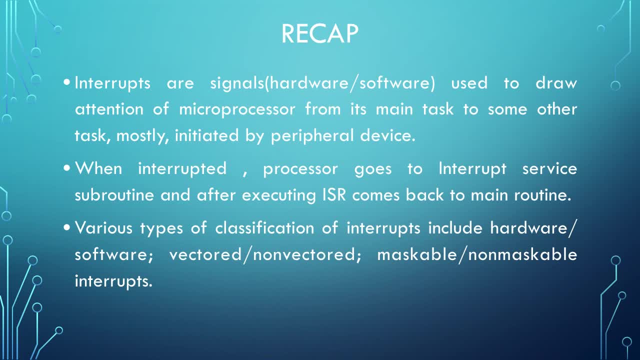 processor from its main task to some other task, These interrupts. Whenever the interrupts Interrupt comes, microprocessor goes to interrupt subroutine and after executing the interrupt, it comes back to the main routine. There are various types of classification of interrupts: hardware, software, vector, non-vector. 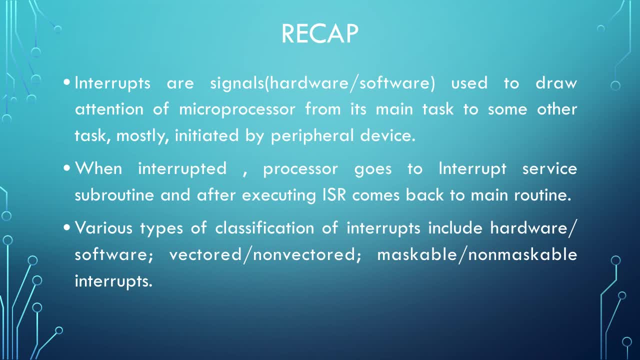 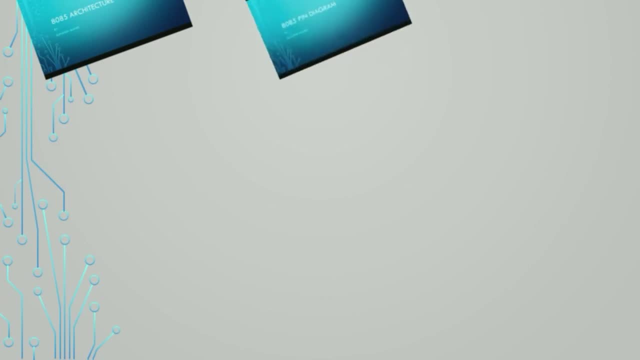 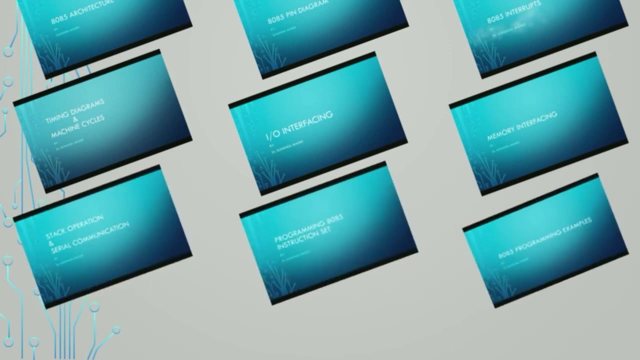 maskable and non-maskable interrupts. So I hope you have understood the basic concepts of the interrupts. There are more videos on 8085 processor on my channel, as shown in this slide, To understand 8085 fully. you can view them all and if you like them you can subscribe.